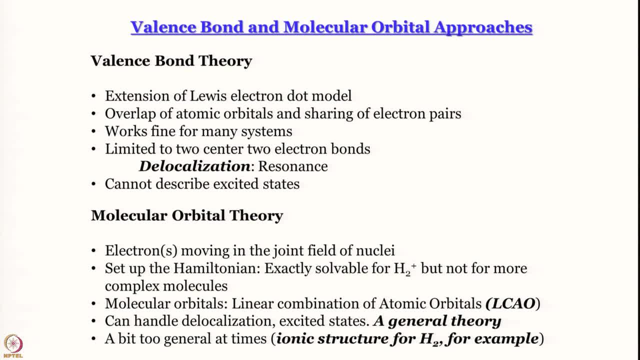 involves molecular orbital calculations. You can use different levels. it is a different issue altogether. But then when we do that, let us not forget our definition of orbitals. An orbital is a one electron system. So when we talk about molecular orbital, what we mean is a one electron wave function for a molecular system. 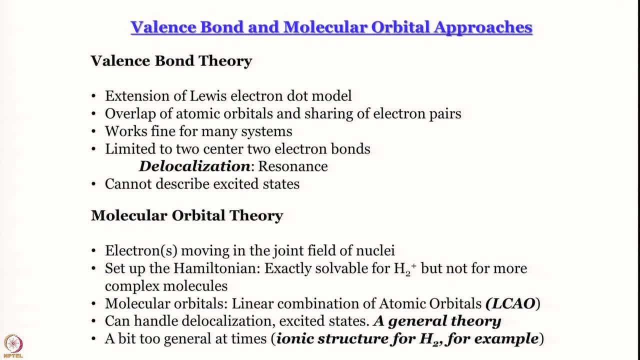 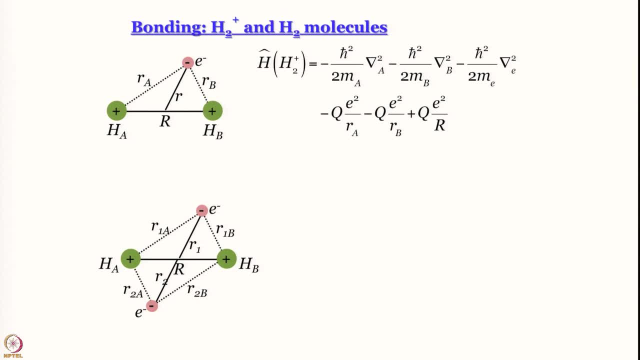 there cannot be any other electron. So what is the simplest molecule that has only one electron and that therefore cannot be handled by ppt? in the first place, That molecule would be H2 plus, And already few classes ago, few lectures ago, we have shown you the Hamiltonian for H2 plus. 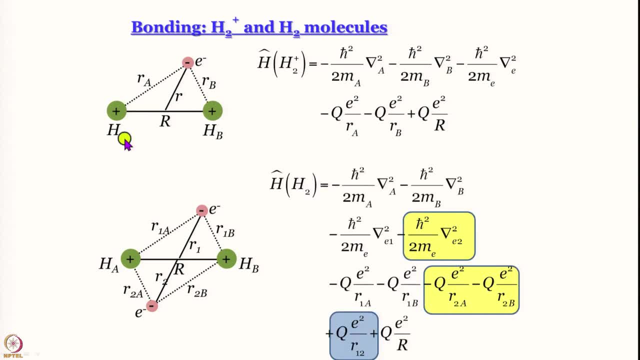 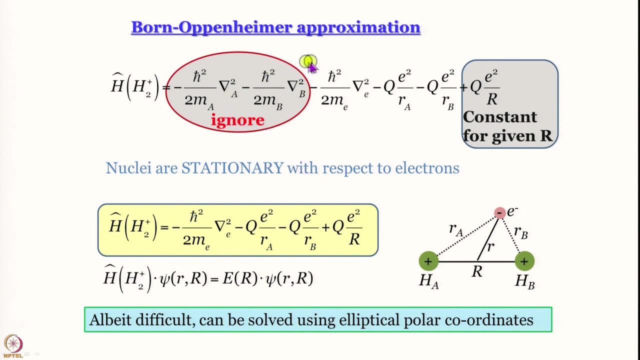 as well as H2.. There are more terms as you go from hydrogen atom to H2, plus to H2. the number of terms keeps increasing as number of as the as different, different interactions come in. Now what we are going to do is we are going to use our good old Born Oppenheimer approximation. 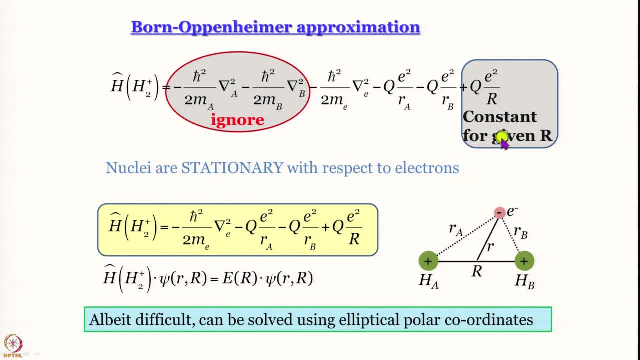 and say that nuclear stationary with respect to electrons. So we are going to hold this capital R inter nuclear separation to be constant for the calculation and we are going to royally ignore the kinetic energy terms for the 2 nuclei. So the Hamiltonian we are going to use really is minus h cross square by 2 m e. 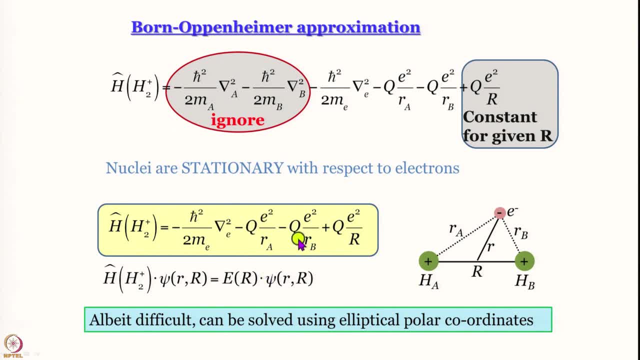 del square minus q e square by r a minus q e square by r b plus q e square by capital R. I am not using atomic units here. We should be equally using atomic units here. We should be comfortable with both. So for a change, let me use this In the next discussion we have. 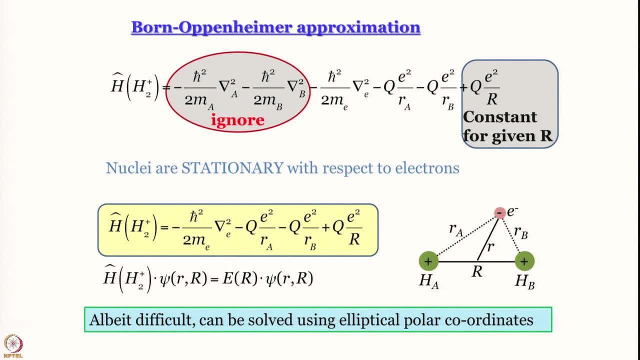 Hooke approximation. perhaps we will use atomic units once again. So this is our Hamiltonian and it is a one electron system. The difference is that, unlike hydrogen atom, it is not a central field problem. There are 2 nuclei, 2 foci, So you cannot use. 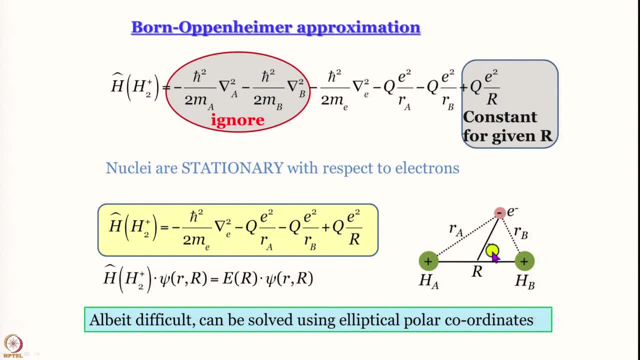 spherical polar coordinates anymore. You can use electrical polar coordinates and you can actually solve, actually get an exact solution. So you can actually solve, actually get an exact solution For Schrodinger equation for h2 plus. but we will not do it. It has been done. I mean there is. 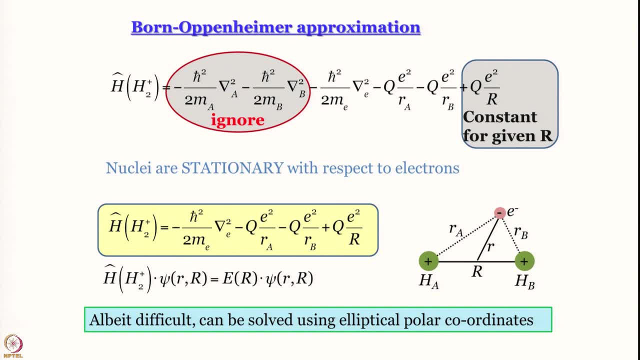 published literature. It is there in some textbooks, but you find that they are there in exotic textbooks. You will not find them in the textbooks that we use- Macquarie or Pillar or even Szabo, because there is no need, Because you put in so much of trouble and 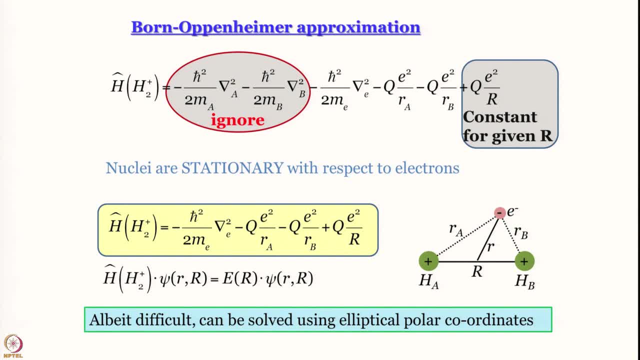 use electrical polar coordinates and get some solution. you cannot use them. You do not know what you are doing. You can bring in one more electron and talk about h2, which is the smallest real molecule. So the thing is this: it is better to start using approximation right away, since you 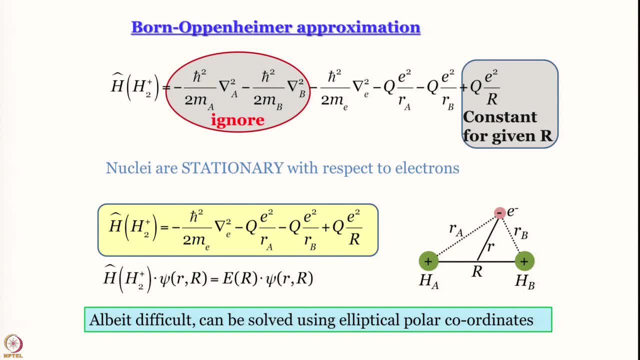 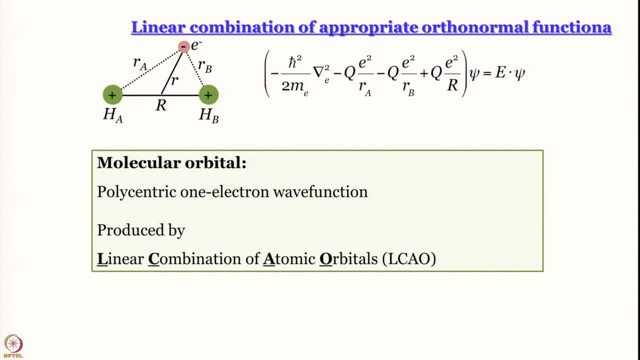 cannot avoid it one step down the line. So the approximation that we are going to use is something we have learned while talking about variation method. Remember we had said that, since, in any case, variation method allows us to change parameters and try and minimize energy with respect to this parameter. 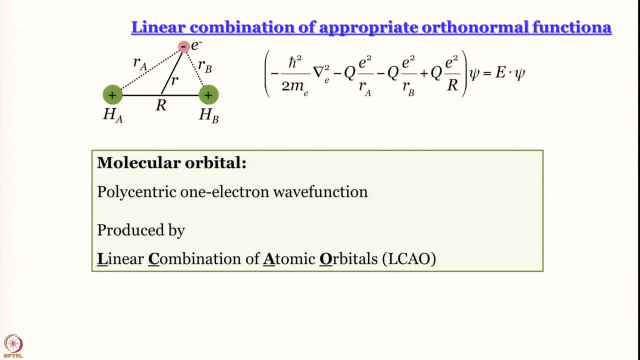 How does it matter what kind of functions we use? You might remember that elephant on the opening slide of a couple of the lectures that we had had some time ago. Those elephants were drawn using some mathematical function. So any wave function, whatever is the real wave function, even though we 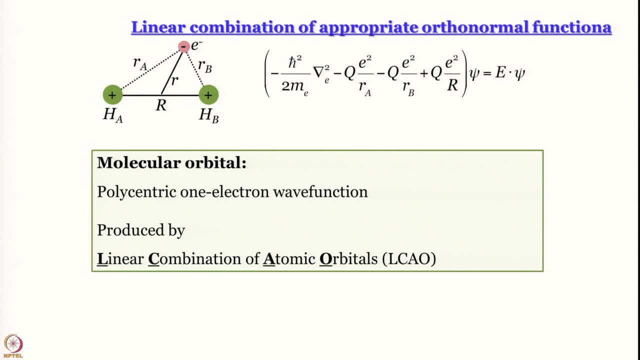 do not want to do it exactly, we can use some sum of Gaussian or Lorenzian or exponential polynomial products of these functions and we can actually simulate these. actually the correct shape, and that is good enough. So if we take an appropriate set of orthonormal functions, orthonormality, 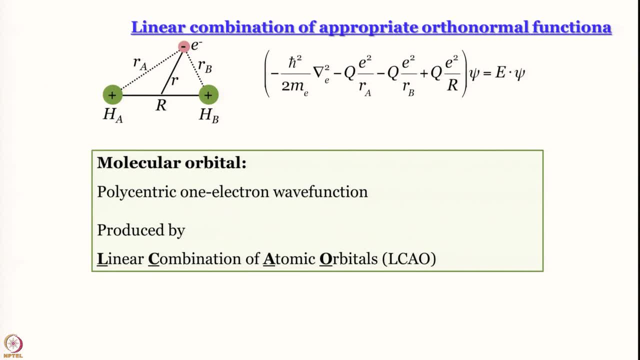 using orthonormal set brings in some advantages, as we have learned in our discussion of many electron atoms. And here the biggest advantage is that we already have a set of relevant orthonormal functions at our disposal, and they are the atomic orbitals. So what we do is we generate the molecular orbitals by linear combination of atomic 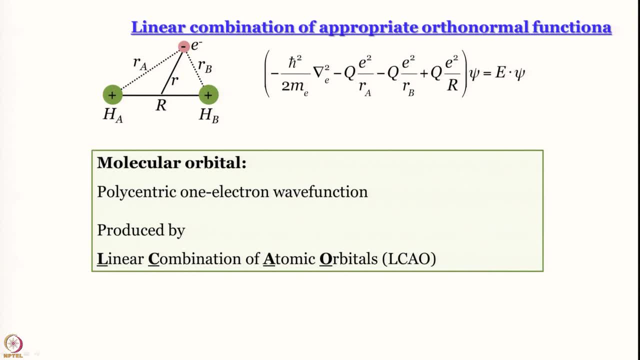 orbitals. This is the first approximation. of course, later on atomic orbitals are not used and molecular orbitals are used by using just what I said: products and sums of different kinds of functions. But for this course we will stick to linear combination of atomic orbitals because 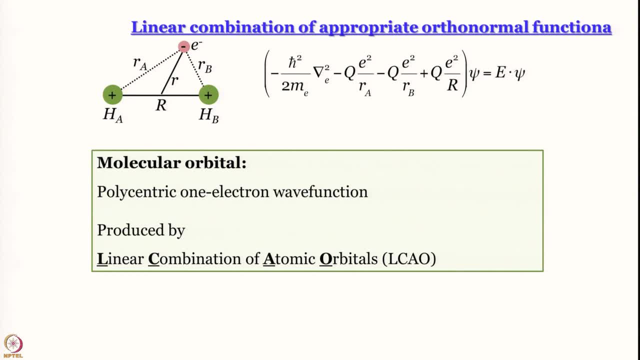 they give us a nice insight of what is going on and it can give us fairly good estimates of energies. Okay, so LCAO, as it is called, is what is going to be used for H 2 plus. the only atomic orbitals that we need to consider are the 1s orbitals. 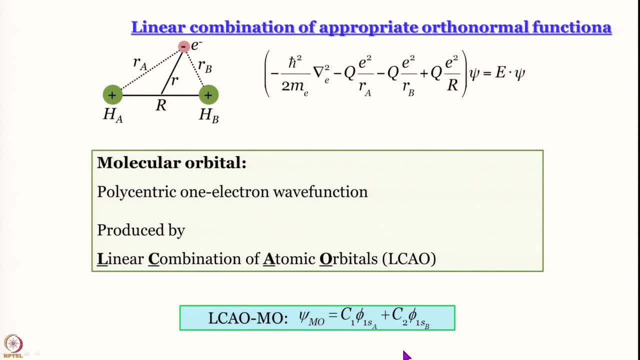 because, ah, where is the electron? electron will be in the lowest energy state and there is an energy gap between 1s and 2s. So this is something where, implicitly, we have used an important principle that is going to come back and get used many times in our discussion, And 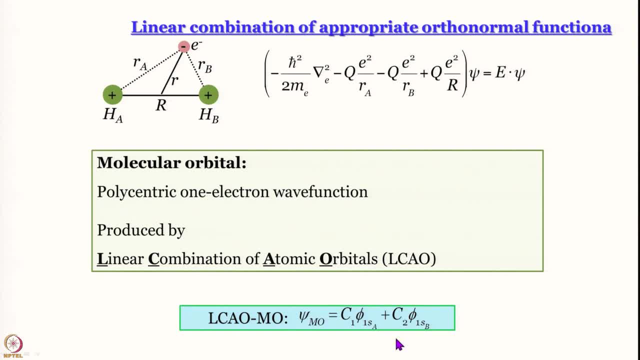 principle is that only orbitals of appropriate energies are going to participate in the linear combination. and later we are going to say: only orbitals that have the correct symmetries will participate in linear combination- Correct symmetry and comparable energies. without that they do not participate in this linear combination. a little bit of difference in energy is okay. 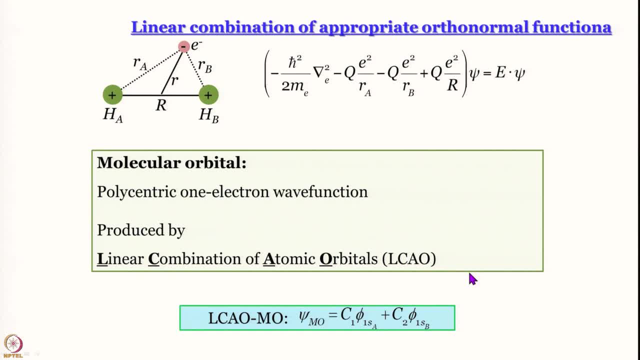 But here the difference would be 1s and 2s. so no, cannot, makes no sense in bringing in 2s. you might get a little bit of improvement if you do, but at our level in this course we are good with this. So the LCO MO we use is C 1, 1s a plus C 2, 1s b, and I hope this reminds you of the wave. 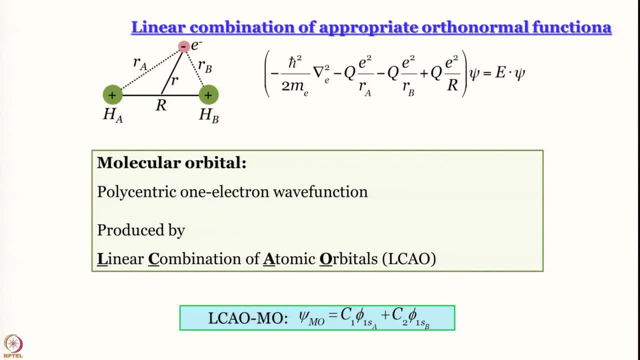 function we had in the valence bond approach. there also we had used the 2 1s orbitals. okay, But the difference there was that we started with filled orbitals. right, we started with 5 1s a 1 multiplied by 5 1s b 2. then to that we added 5 1s b 1, 5 1s b 2, and then we proceeded. 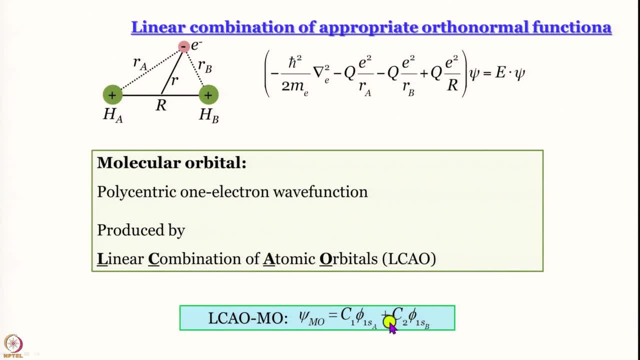 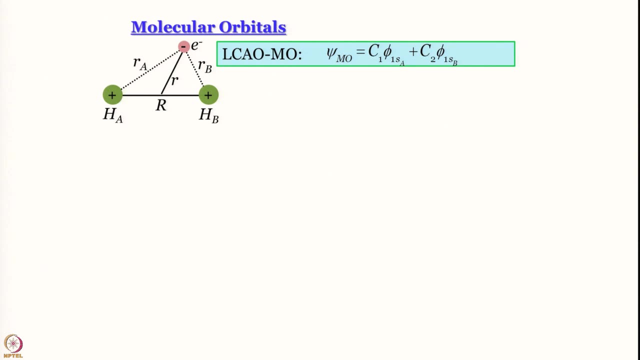 Here we do not bother about the electron to start with. we are more interested in constructing the wave function, and then we will fill in the electron when it is appropriate time. But let us work with the, with this molecular orbital, to start with C 1 1s a plus C 2 1s b. so 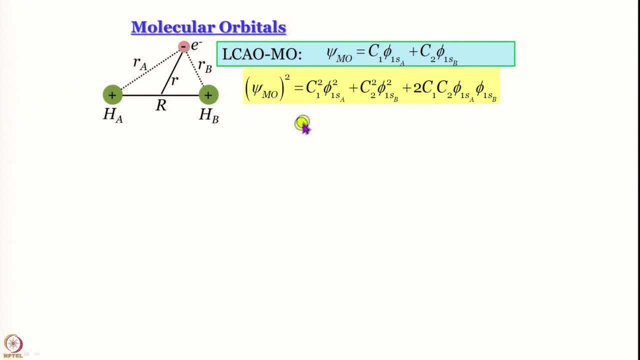 take square of that, this will give you probability density. that is C 1 square 5 1s a square plus C 2 square 5, 1s b square plus 2 C 1, C 2, 5, 1s a, 5 1s b. Now see, is there any reason why in these two 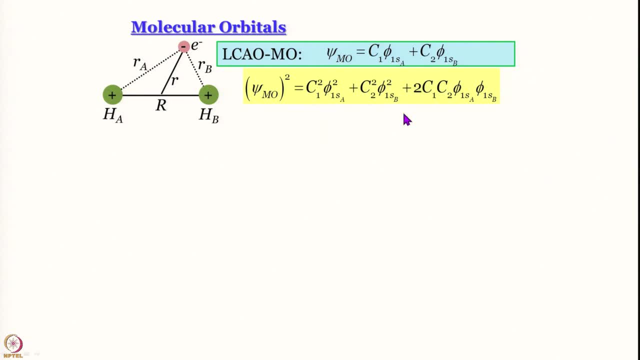 terms, C 1 square should be different from C 2 square. we had used exactly similar argument for valence bond theory. also No reason why any of these 2 orbitals will make a different contribution. so it makes sense to say that C 1 square equal to C 2 square, or C 1 equal to plus minus C 2. okay. 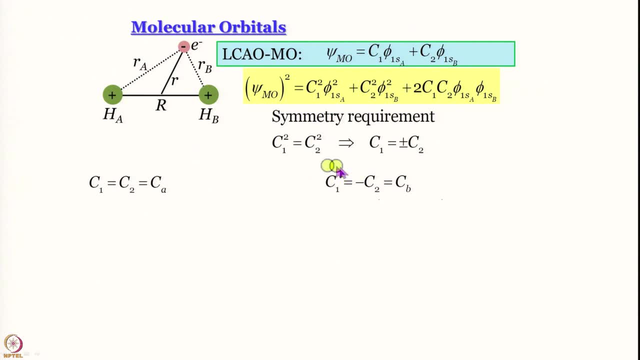 So that we can write: when C 1 square equal to C 2 square, when C 1 equal to C 2, we write C 1 equal to C 2 equal to C a, and when C 1 is equal to minus C 2, then we equate it to. 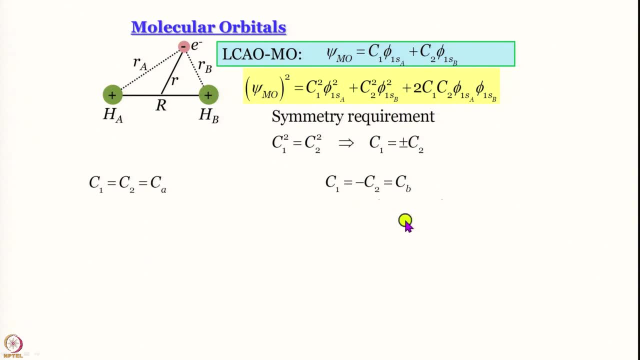 C, b. Of course this is a bad choice. well, I should not say of course. actually it is a bad choice because it is better to write B here and A here, for reasons you will see very soon. All right, so what is the wave function then? the wave function, the first wave function where we 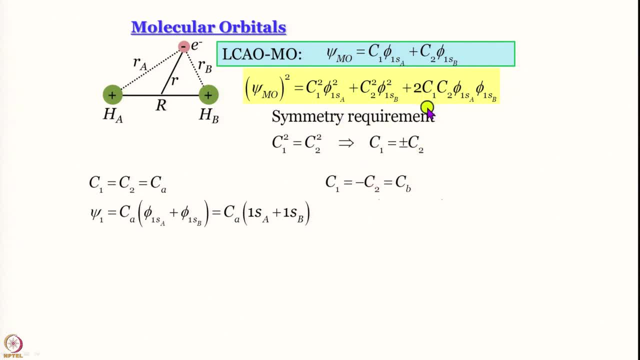 use a linear combination with plus sign is C A multiplied by phi 1 S A plus phi 1 S B. So in the subsequent discussion most of the time we have not written phi, we have simply written 1 S A plus 1 S B. what about Psi 2? Psi 2 would be C B into 1 S A minus 1 S B. 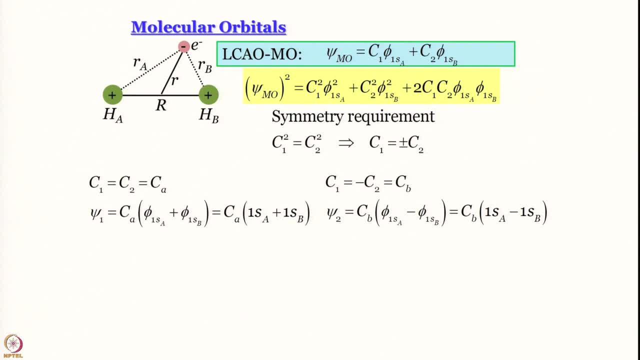 and I think most of you would know already that this plus combination is a bonding orbital. this minus combination is the anti bonding orbital. why bonding? why anti bonding will come to it in its time, But now this is what we have Generally. we like to drop. 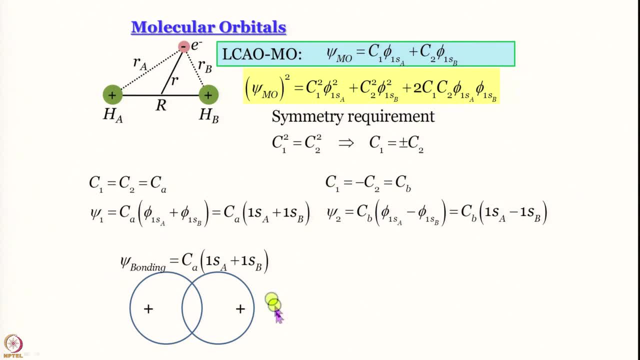 pictures instead of writing algebraic expressions, and this is a picture that we generally draw. we draw two circles for the two S orbitals and we would put two plus signs to denote that the combination is plus and for anti bonding, we put a minus sign in one of them. 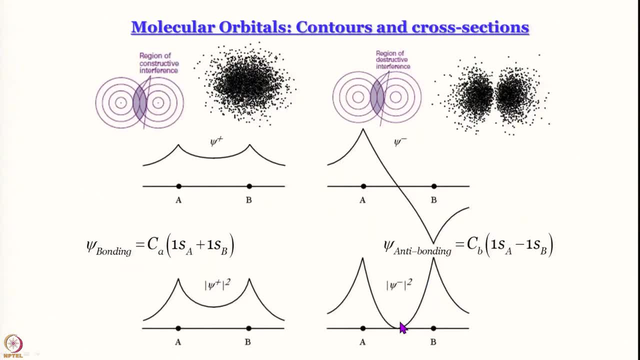 to denote that the combination is minus. In fact, it is better for us, since we know about contour diagrams and all. we can look at the contours and understand better. these are the overlapping contours of A and B orbitals. here, the only difference is that you have to put in the plus and minus sign and you 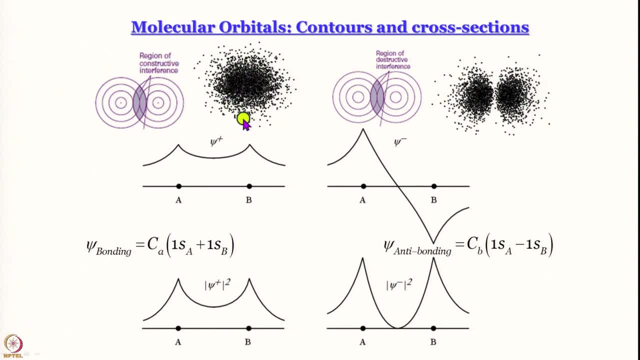 can draw this Psi square like this: as dots, remember, we put a dot wherever there is some probability, so we can generate the diagram of Psi, Psi, star, Psi square. it will be like this: no node here. here there will be a node because in this region there is going to be. 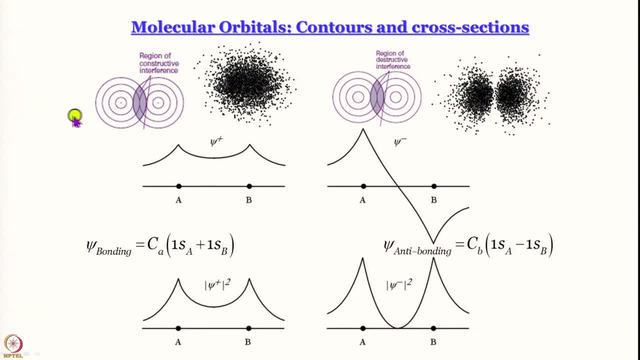 a destructive interference. so if you look at, look at the profiles, take a cross section of this orbital, you will get two peaks For Psi plus the bonding orbital. here, however, one S orbital points up, the other one S orbital points down. this is plus, this is minus, remember. so you are going to get a node, a zero crossing. 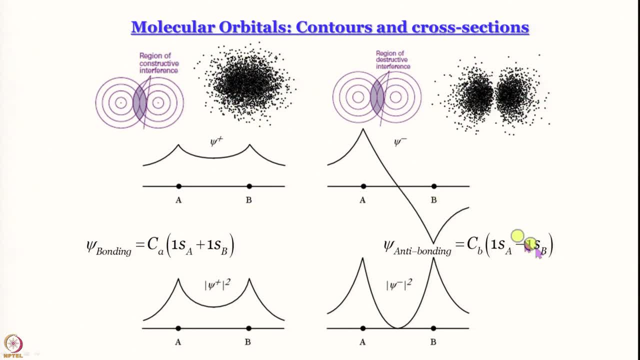 point exactly between the two nuclei, and if you take this Psi square, then Psi square looks like a circus tent in case of the bonding orbital and it looks like two circus tents right beside each other For the anti-bonding orbital. so, ah, generally, what ah the argument that is given in many 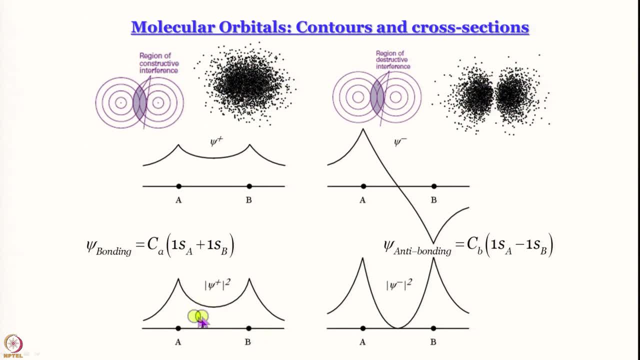 textbooks, even though it is not. it is a little bit of hand waving argument that there is an buildup of electron density because Psi, Psi square is more Psi square, dr will also be more here. build up electron density between the two nuclei A and B and that is why the 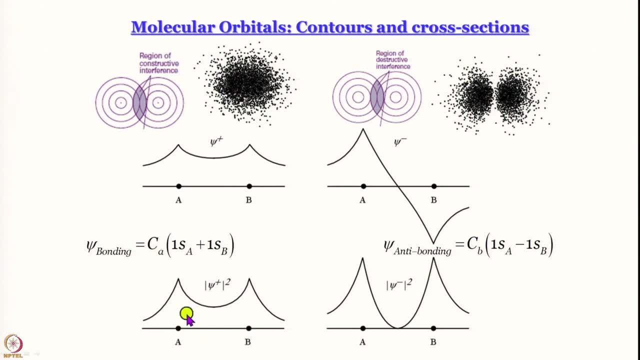 electron sort of shields the two nuclei from each other and act as a cement for them. here actually there is A decrease in electron cloud. if you just do 2: 1 s orbitals and if there is no ah bonding at all, then the picture would have been something like this. I will draw normalized picture it. 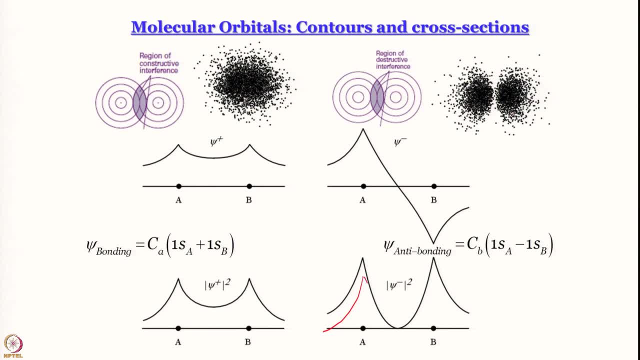 would have been something like this. so in this region you would have this much of electron density more than what you have for the anti-bonding orbital. So generally, even in class 11, 12 books, this is the explanation that is given, So we will. 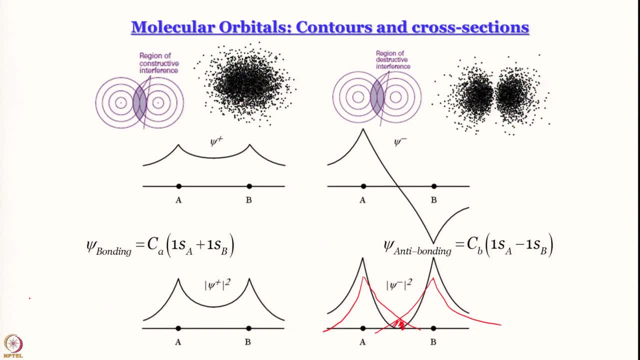 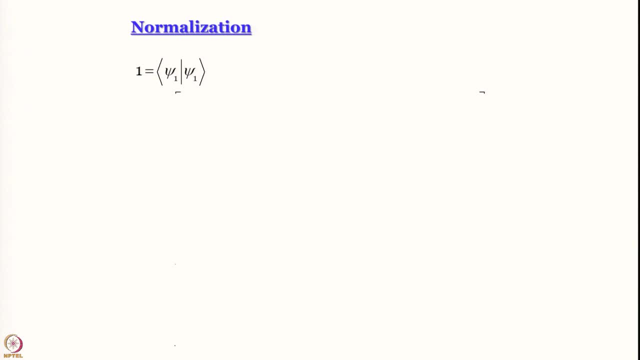 not worry about that explanation for the moment. just go ahead and see how it pans out. To start with, let us normalize this wave function. we know that this is what we usually like to do first. So integral psi 1 squared dr, in this case, will be equal to well, will it? 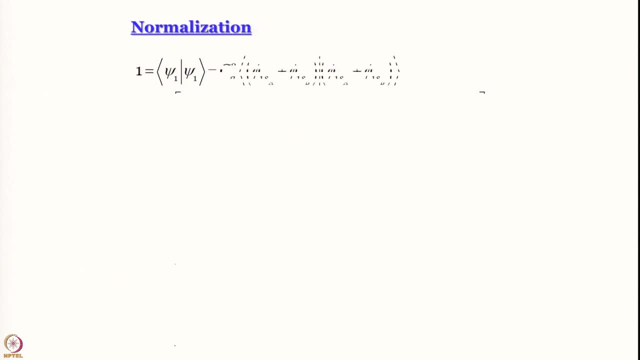 be dr. it will be dr 1, dr 2. right, there are is a double integral again that will be equal to 1.. So you write this. I am going very fast here, because this is more or less what we have done in the valence bound theory approach as well. So expand this. you get 4 terms and 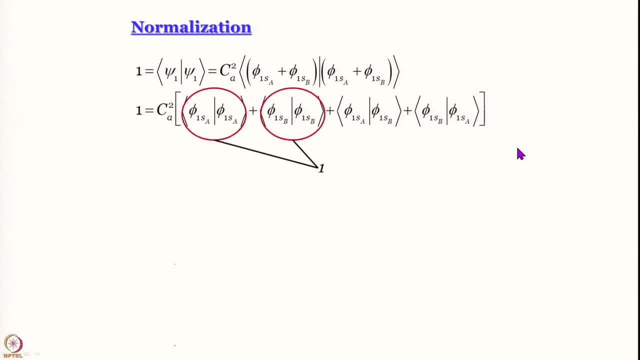 when you look at the 4 terms, they are familiar. Integral phi 1 sa. phi 1 sa dr a is equal to 1.. Because 1 sa is normalized, same is true for 1 sp. and what is this? integral 1 sa, 1 sb d. 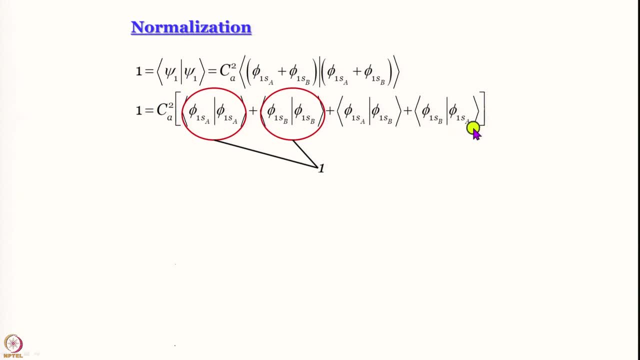 tau integral. 1 sb, 1 sa d tau. you might remember from our valence bound discussion that these are overlap integrals. Remember overlap integrals. these are simply overlap integrals. So what do you have? you have 1 equal to c s squared multiplied by 2 plus 2 s. 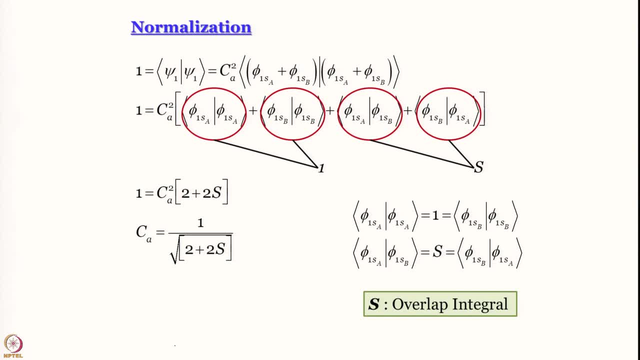 So t a turns out to be 1 by root over 2 plus t s, 2 plus 2 s. Similarly you can find the expression for c b. that is equal to 1 by root over 2 minus 2 s. I am going at breakneck. 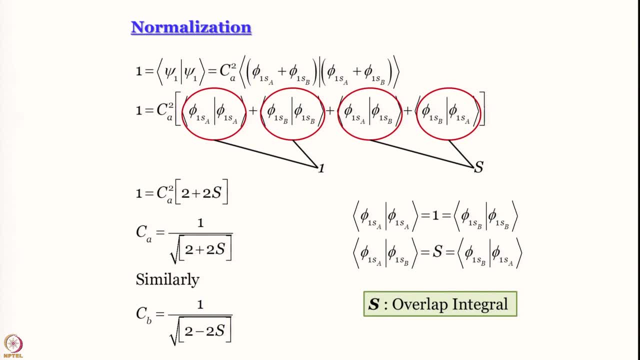 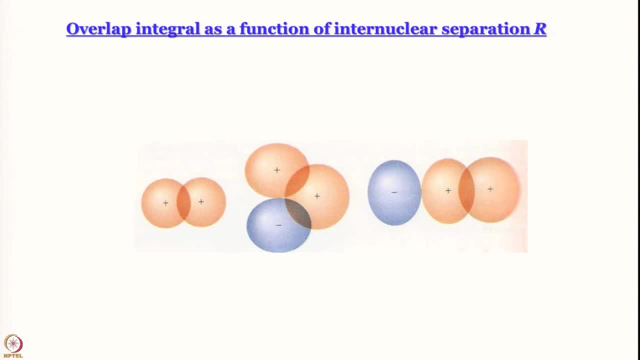 speed, because it is so simple. please work this out yourself, then only you will understand fully. good Now you might remember that overlap integral is actually a function of inter nuclear separation. We have done at least one of these. this one we have done, in fact, for that we had given. 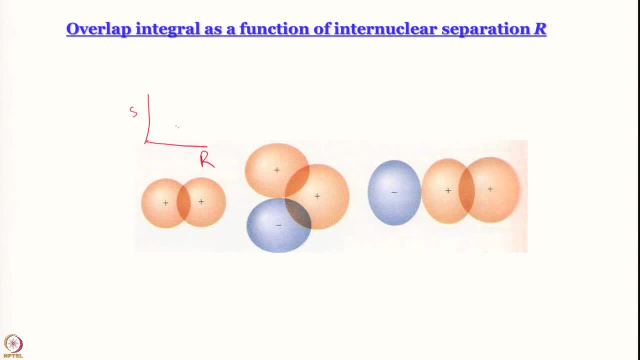 you an expression and we had shown you the plot. and it is not very difficult to see that, when these 2 orbitals are infinitely far away, overlap. integral is of course 0. It comes closer, overlap will go up, up, up, up up and finally it will be something like this: What? 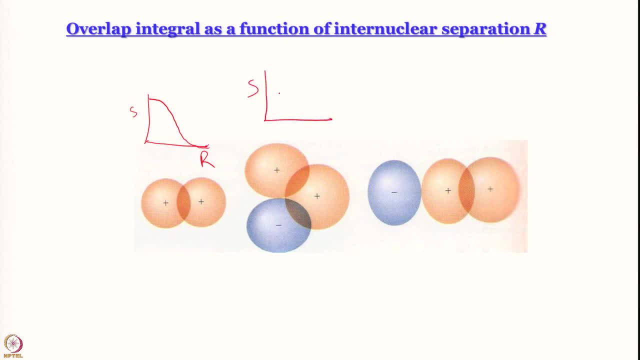 about this? This is a very curious case. Overlap integral when the overlapped integral is of course 0.. What about this? This is a very curious case. Overlap integral when the overlapped integral is of course 0.. What about this? This is a very curious case. Overlap integral when this r equal to infinity. 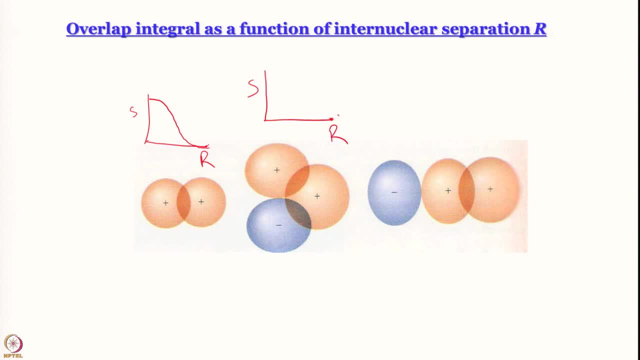 is of course 0.. Now, even in this case, what is the overlap integral? Is it 0 or is it something else? Do not forget what overlap integral is. you have to do a point by point multiplication of the 2 wave functions and add. So this is 0. So this is really an. 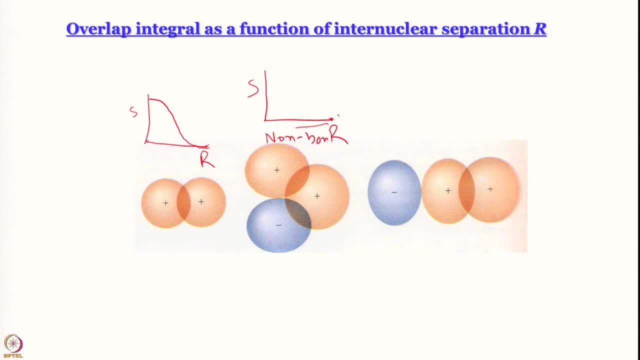 example of non bonding interaction Here: when you have sigma interaction between the two wave functions and add, So this is 0. So this is really an example of non bonding interaction Here. when you have sigma interaction between an s and a p orbital, then what will the overlap integral? 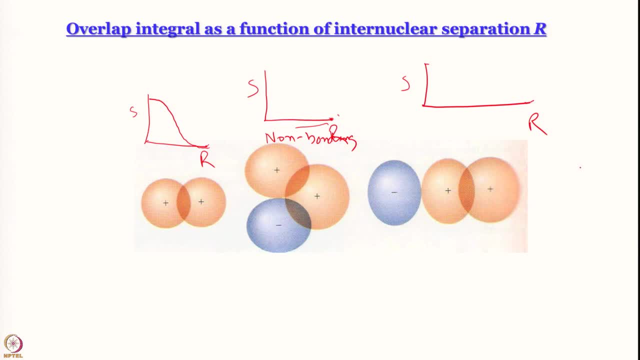 be like 0 here. and then, when I bring this close together, say this is your p orbital minus plus, change color and this is your s orbital plus. Now what happens? Is it 1? Is it 0? what is it? for? this part is going to be plus, for this part it will be minus and the 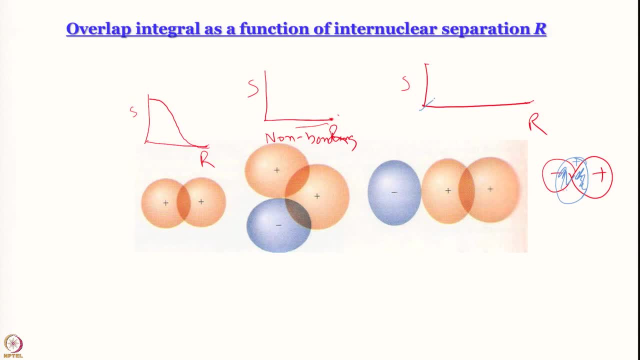 magnitude is same. So it is going to be 0 at r equal to 0, 0 at r equal to infinity. somewhere in the middle it is going to peak. where will it peak? it will peak in the situation where this s orbital is here. that is where it is going to peak. So for inter nucleus separation, here to 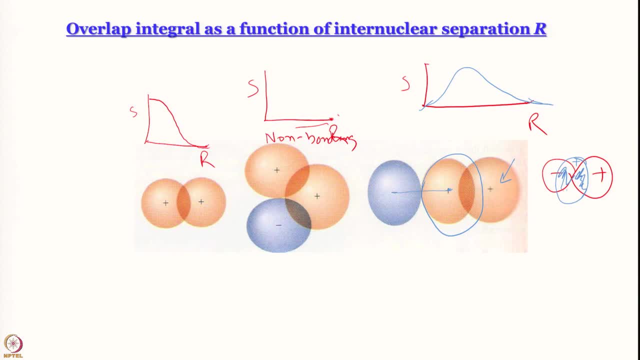 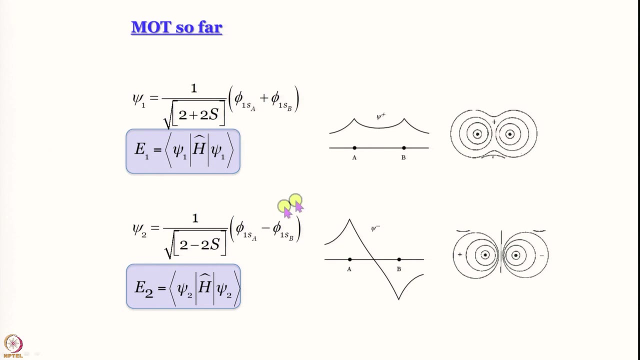 let us say here: So in our tutorial, we have some problems in which you have to work this out. I think you have- you might have done it already in our assignment- great. So this is what we have. we have an, we have expressions for the. 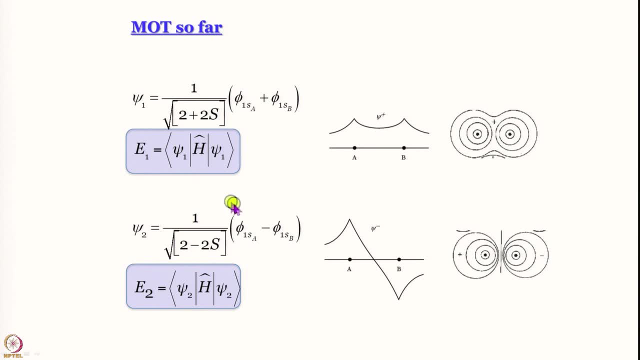 bonding and anti bonding orbitals. that is great, and now our job is to find the expression for energy expectation, value of energy by using these wave functions for bonding and anti bonding orbitals. We will call the energy of the bonding orbital E 1, bonding MO E 1 and we will call the 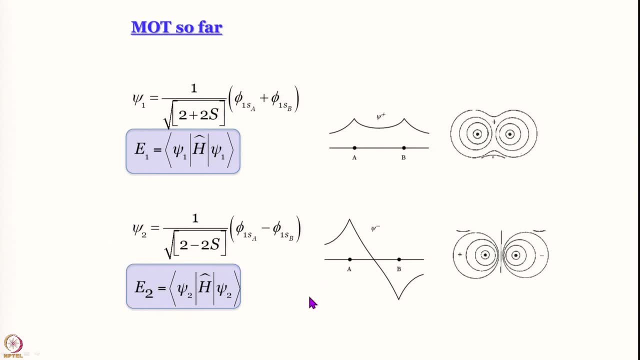 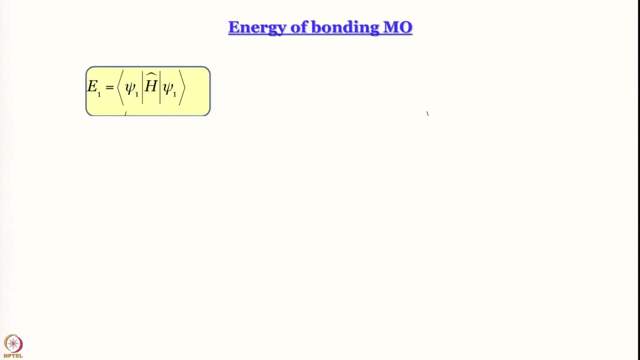 energy of the anti bonding MO E 2. well, it is perfectly okay to call the MO s orbitals. they are orbitals, but I prefer to call them MO s because we are also using atomic orbitals, and by an orbital. So by now we have become used to referring to atomic orbitals as just orbitals. okay, now let us. 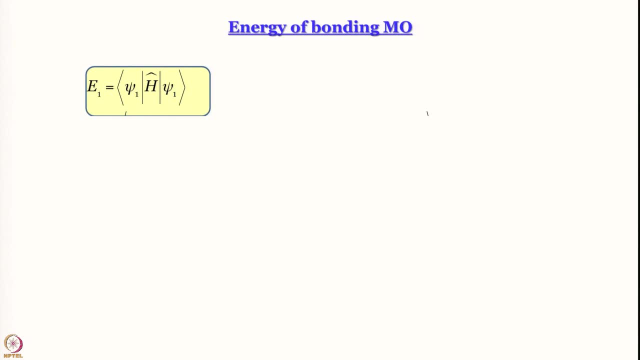 see what the expression for energy of bonding MO would be. and once again I am going fast because this is now cakewalk for us, right? what is this integral? first thing to do is plug in the value of psi 1 and take out the product of the normalization constant. this is what we get. E 1 is. 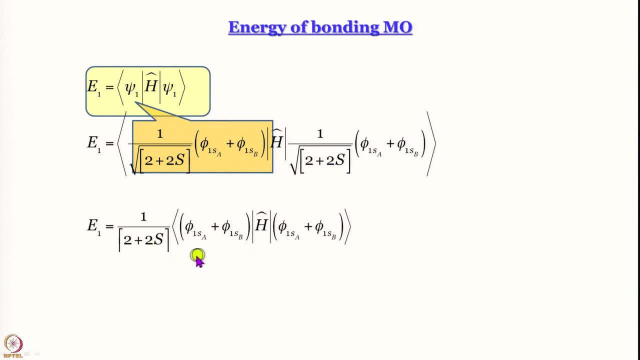 2 plus 2 s multiplied by. in bra vector we have phi 1 s a plus phi 1 s b. in the ket vector we have h hat, 1 s a plus 1 s b. Of course you should expand and you are going to get 4 terms. 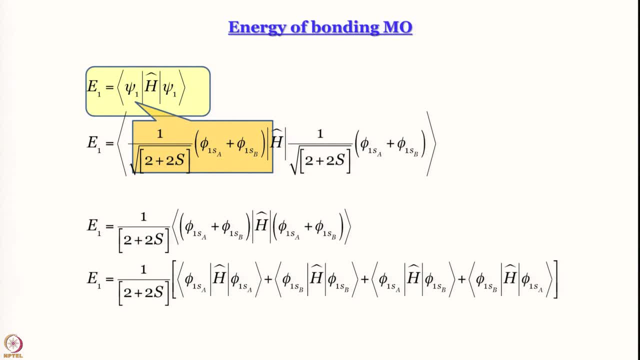 and the 4 terms, I hope, do not look absolutely unfamiliar to us. Similarly, we can get an expression for E 2, and point to note is that if you look at E 1 plus, plus, plus, well, of course this is also plus for E 2. the integrals remain the same. 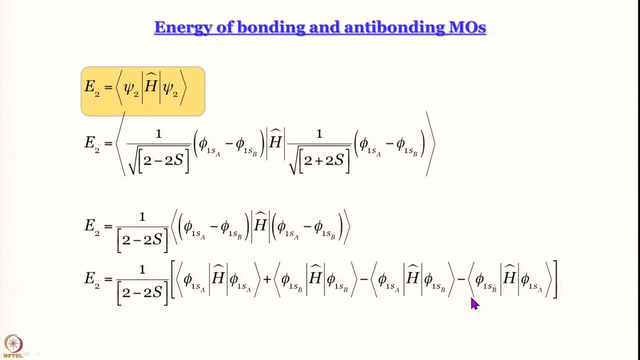 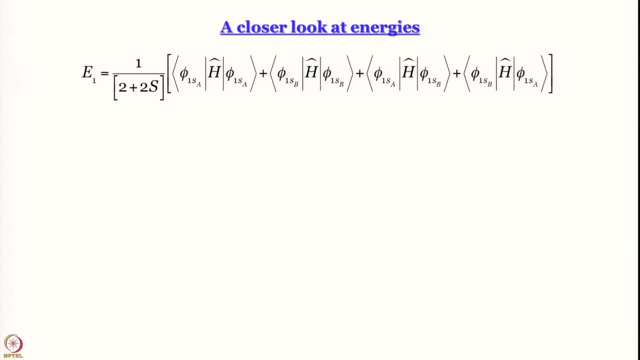 only in these 2 cases plus becomes minus. there is no other difference. Now let us take a closer look at these energies. ah, do we know these integrals? have we encountered integrals like this? ah, integral phi s a h hat phi s a. well, phi 1 s a. 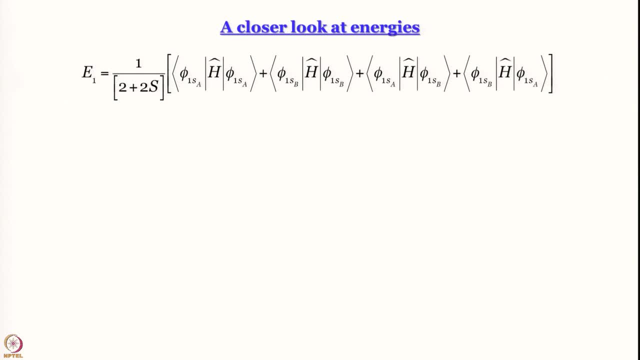 h hat phi 1 s a. h hat phi 1 s a. Integral psi i. h psi i. what is? it? is not it? h i. integral phi 1 s b. h hat phi 1 s b. again, that is h i i. you can call it h j, j, but they are the same, does not matter. 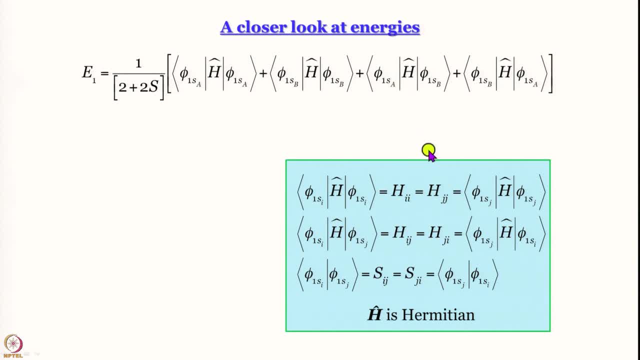 Integral phi 1 s a. h hat phi 1 s b. what is that is s i, j and integral phi 1 s b? h hat phi 1 s a is s j, i, but then s i and s j are equal because, if you remember, h hat is a Hermitian and so we can use turnover rule. 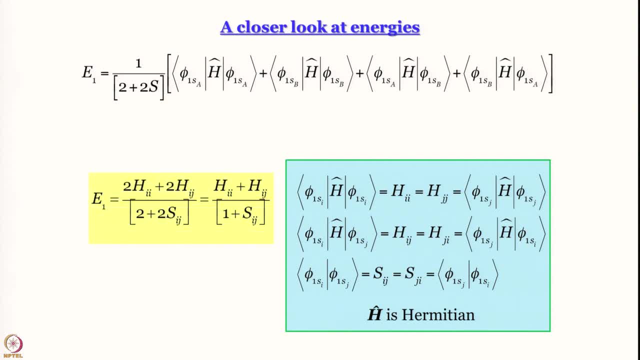 So these are familiar integrals for us. we might as well write E 1 in terms of h, i, i, h, i, j, and for now we will write s i j, and whenever we are bored of writing i j, we are going to go back to s, does not? 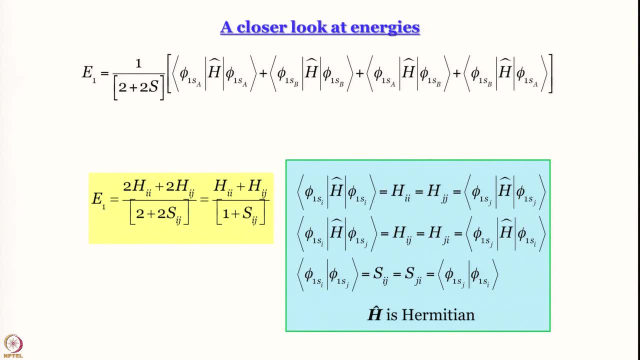 matter. So E 1 turns out to be h i i plus h i j, divided by 1 plus s i j. you might as well write h 1 1 plus h 1, 2.. Does not matter, perhaps it is better to write h 1 1 plus h 1, 2.. What about E 2?? In E 2, if you. 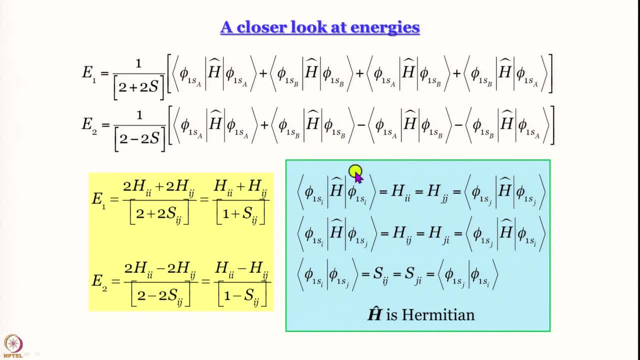 remember the only difference was that the last two terms had minus, negative coefficients, negative signs. So plug that in. you get E 2 to be h i i minus h i j, divided by 1 minus s i j, both become minus. So now to go further. we need to evaluate h i i. we need to evaluate s i j. we already know what s i j is. 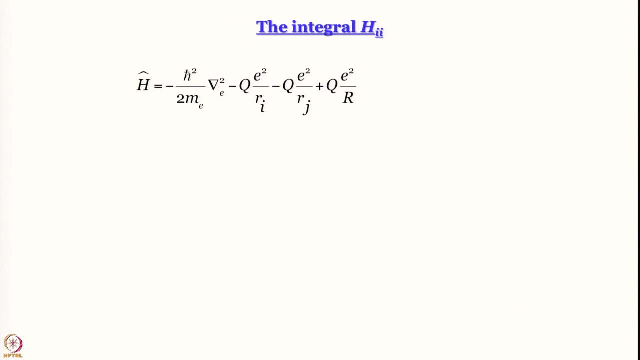 In fact we already know what h i, i, h i, j are as well. we are just revising. So this is your Hamiltonian, this time not in atomic units. minus h cross square by 2 m e del square. minus q r square by r i. you can recognize that these two terms constitute a one electron wave function, minus q e. 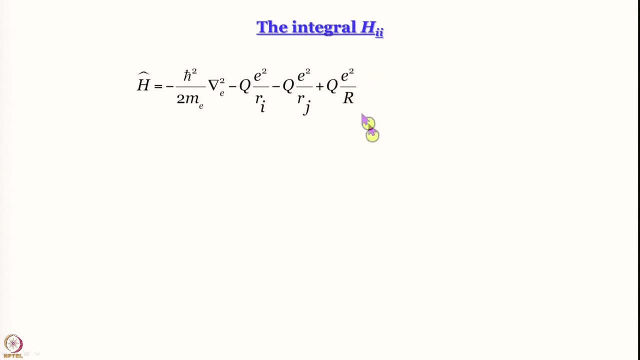 square by r, j plus q e square by r. this is your. this is for the potential energy for attraction between electron and nucleus. Sorry, sorry, sorry. what did I say? q e square by capital, R is for internuclear repulsion, nucleus, nucleus repulsion. So we will club these two together and we are going to write Hamiltonian. 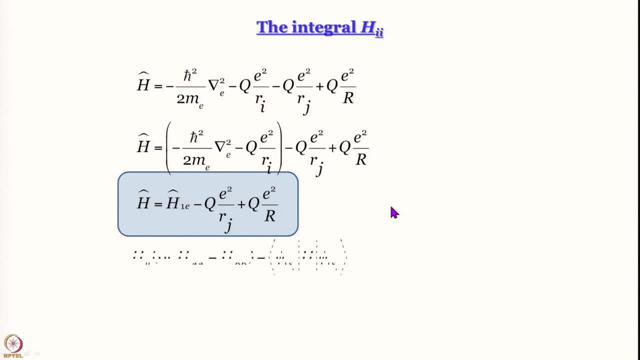 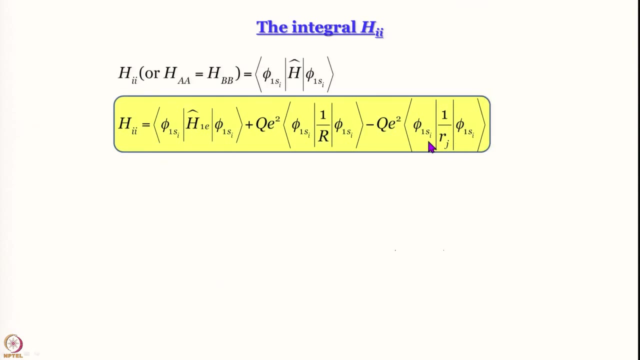 of one electron. So now our Hamiltonian has three terms. So h i- i is integral, phi s i left multiplying Hamiltonian operating on phi 1 s- i. So we will write like this: okay, same expression. so no harm done: h i- i equal to sum of these three terms. 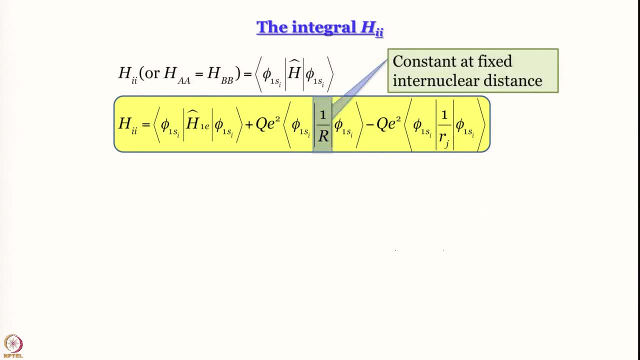 Now look at this: 1 by r is a constant at a fixed inter nuclear distance. right we? we are working under the ambit of Born-Oppenheimer approximation. Here I might digress a little bit and I might say that the Born-Oppenheimer approximation 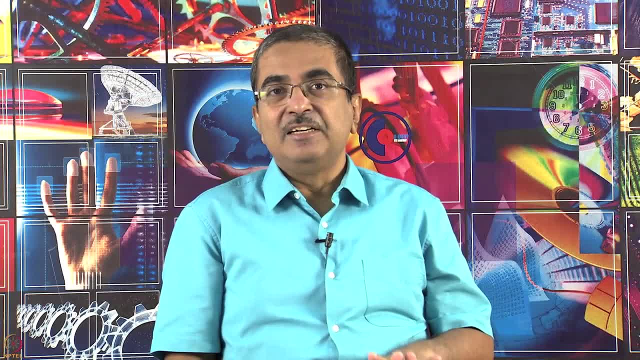 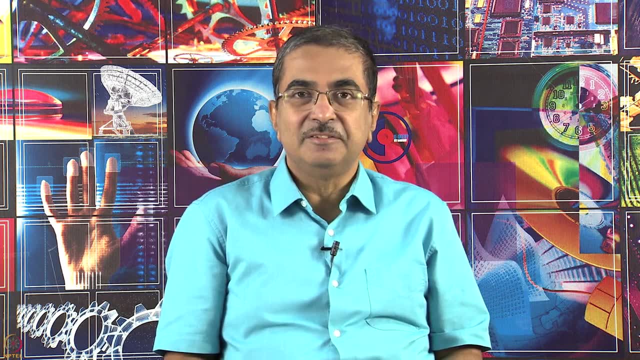 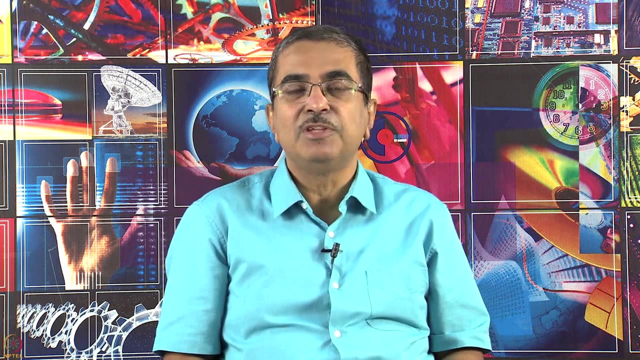 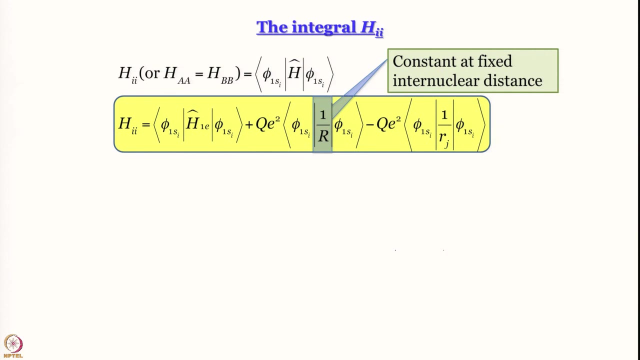 does not hold in all cases, but that comes under the beyond approximation theory limit. that is a little more complicated phenomenon. for our purpose, Born-Oppenheimer approximation is actually a very good approximation. we can work without its ambit without losing general life generality. So this is a constant at fixed inter nuclear distance. fine, so we can bring it out. what did I do? 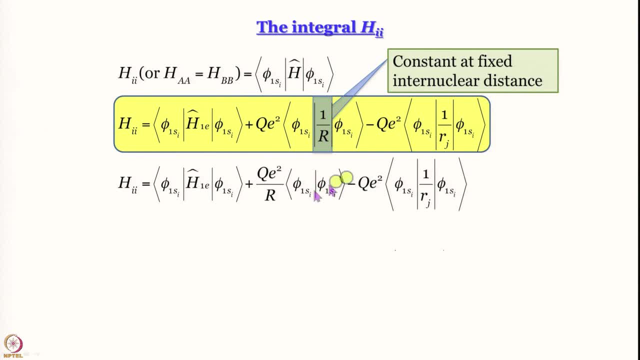 sorry, So I can write like this: integral phi 1 s i h 1. electron phi 1 s i. we will come back to this- plus q square. integral phi 1 s i. phi 1 s i minus q square q square. integral phi 1 s i 1 by r j phi 1 s j. Again, I hope that these terms do not. 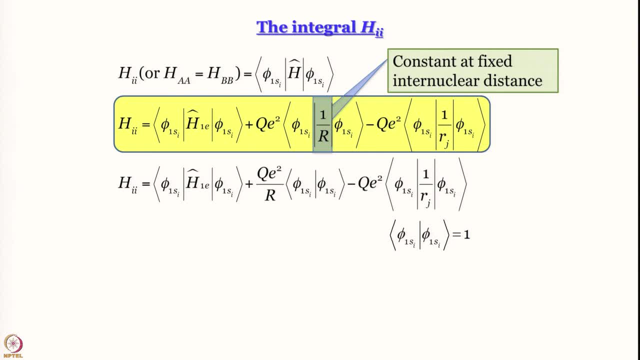 look unfamiliar to you because, first of all, phi 1 s i, phi 1 s i, integral of that. what is that? that is simply 1. it is normalized integral of phi 1 s i into 1 by r j phi 1 s i. what is that is? I hope you. 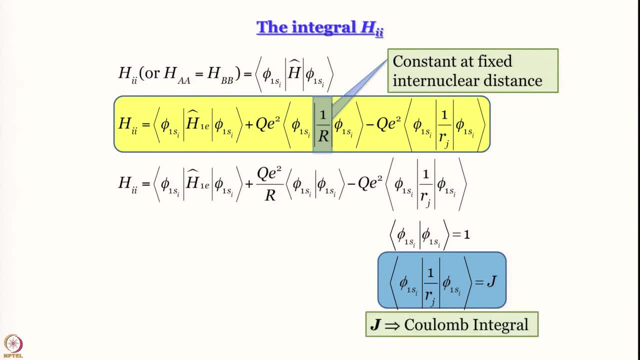 remember that it is the Coulomb integral. j remember Coulomb integral. Coulomb integral denotes the electrostatic interaction out when we talked about dihydrogen molecule in your valence bond theory And I hope it is not very difficult to see that integral phi 1 si h hat 1 electron phi. 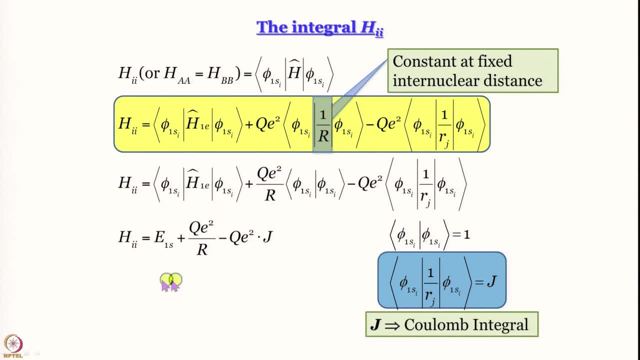 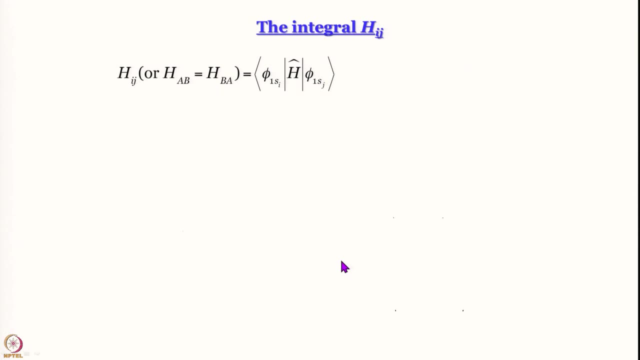 1 si. what will that be? h hat, that will be the expectation value of energy of 1s orbital. it does not matter whether I use a or b. this energy of 1s orbital is still the same. So energy of 1s orbital plus q square by r, minus q square into j. Now let us evaluate the integral. 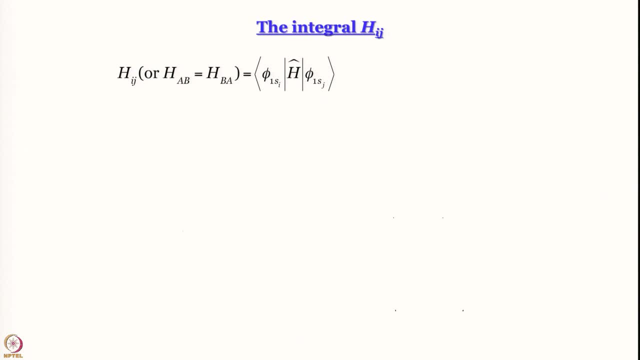 h ij. it is not enough to evaluate h ii. I want energy finally, So h ij. similarly, we can proceed and we can again use this 1 by r to be constant. h ij will be first of all. this is the value of h ij. So this is the value of energy for your 1s orbital. then q, square by capital R, as we know. 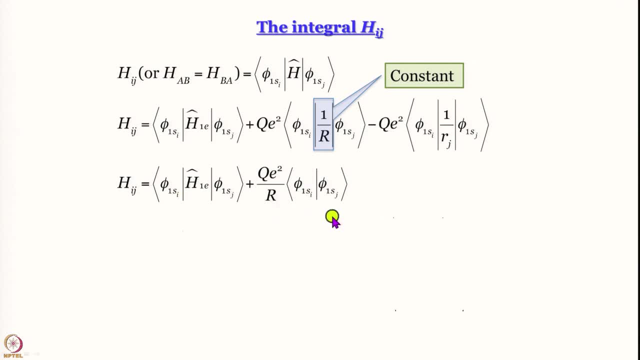 that this, ah, what is this? integral of 1 si 1 sj. what is that going to be? that is going to be s right overlap integral will not be 1.. And this integral minus q square integral phi si 1 by rj phi sj. what is that? we know that also right. So the first term is E 1s. 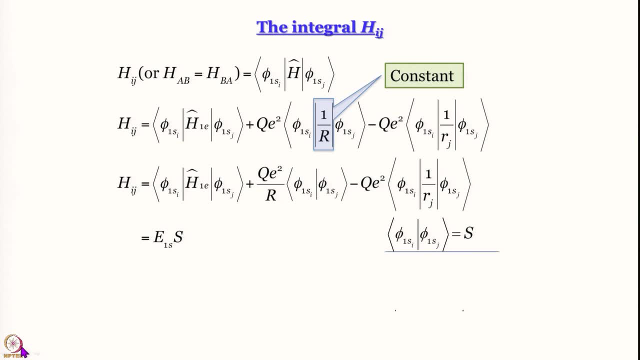 into s. let me that. let me. Let me work that out, because I think I made a careless statement just few minutes ago. I am working this out. what is it? h hat 1 electron operating on phi s j gives me E 1s. So if 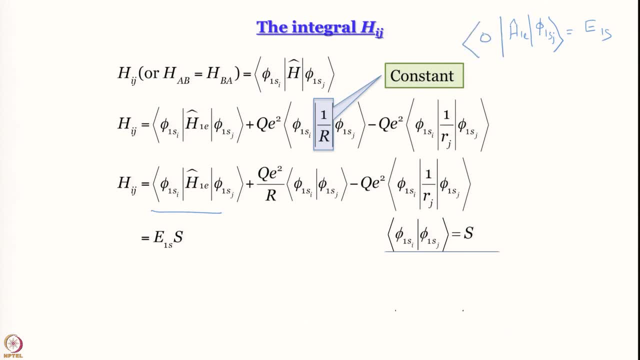 I write it in bracket notation. we have in bra vector phi 1s i. So what will I get? this becomes E 1 s multiplied by phi 1 s j, of course. So you take this and plug it in and, moreover, you take this E 1 s out. you are left with E 1 s multiplied. 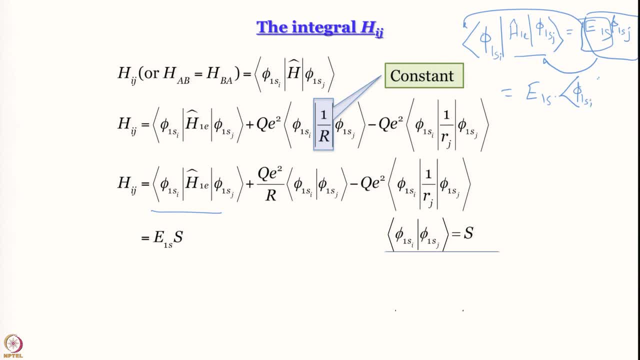 by integral phi 1 s, i, phi 1 s j, that is your s E 1 s s. Next one will be Just q e square by r, multiplied by s same s. is there then? if you look at the third integral, it is k, is not it exchange integral, or I did not tell you this name earlier? it is also 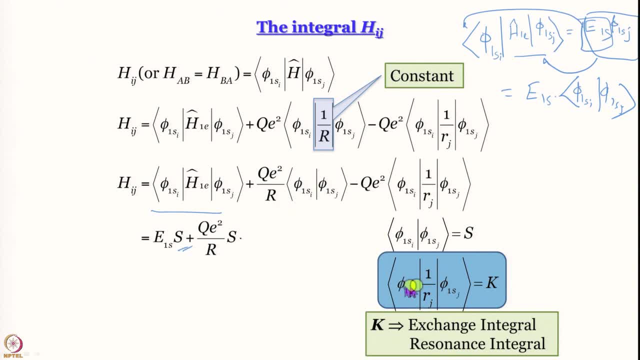 called resonance integral, because here you are considering 1 s i and 1 s j in the same integral, So exchange. so please remember. we will come back to that later. but let us write like this: minus q, e square into k, And remember that k is a purely quantum mechanical concept. there is absolutely no classical counterpart. 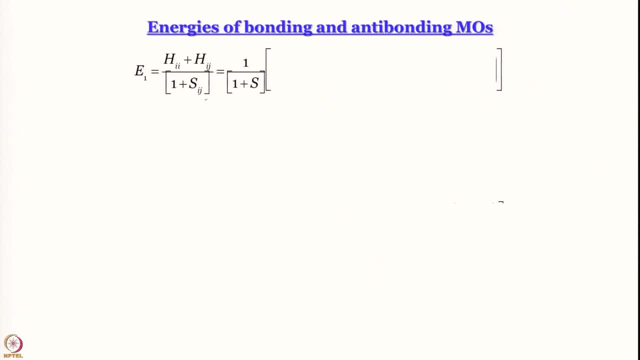 for k fine. So we know h i I, we know h i j. we of course know s i j. it is equal to s. So I have written s i j, equal to s here. Now let me plug in the values of h i i. this is h i i. I hope you. 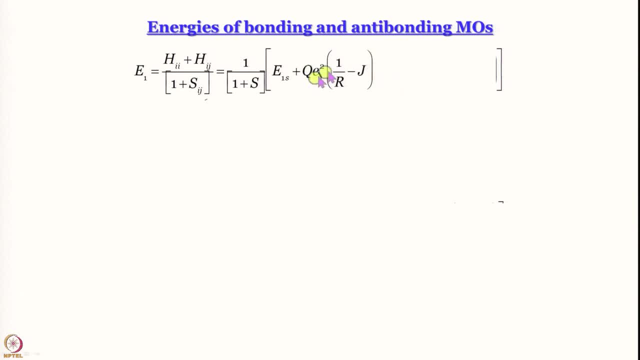 recognize E 1 s plus. I have taken q E square, common q e square multiplied by 1 by capital r minus j. Hey, H, ij is E 1 s plus Q e square multiplied by s, by r minus k, So E 1 will then be equal. 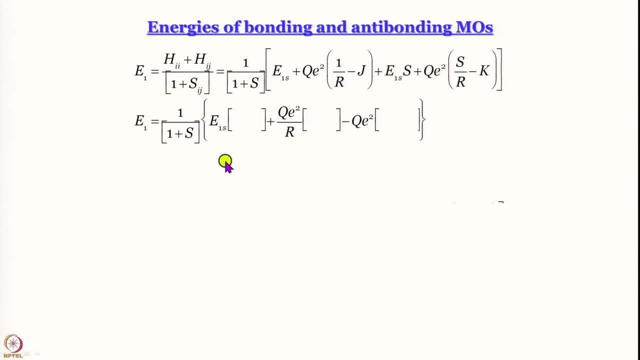 to if I now collect the coefficients of E 1 s, Q e square by r and minus Q e square. So what will be the coefficient of E 1 s, E 1 s into 1 plus s, is not it 1 from here s? 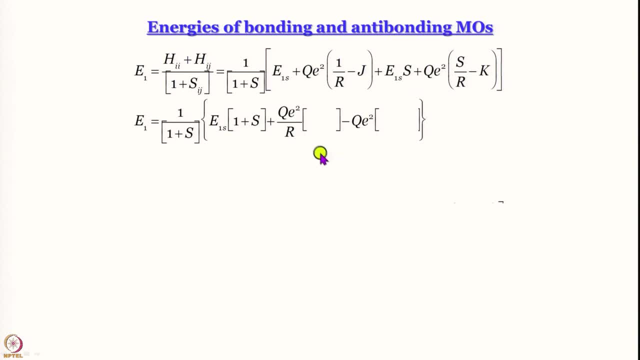 from here. what will be the coefficient of Q e square by capital R, Q e square by capital R, so 1 from here and s from here. so 1 by s minus Q e square. what will be the coefficient? you take minus outside from this term, you get J. from this term you get k minus Q e square. 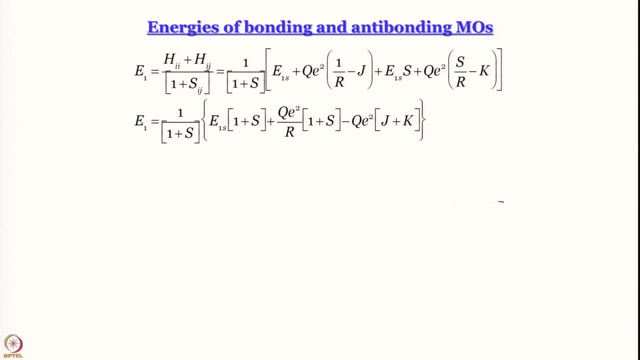 multiplied by J plus k, That is E 1. so E 1 then turns out to be: you just simplify, divide throughout by 1 plus s. you get E 1, s plus Q e square by capital, R minus Q e square multiplied by J plus k. 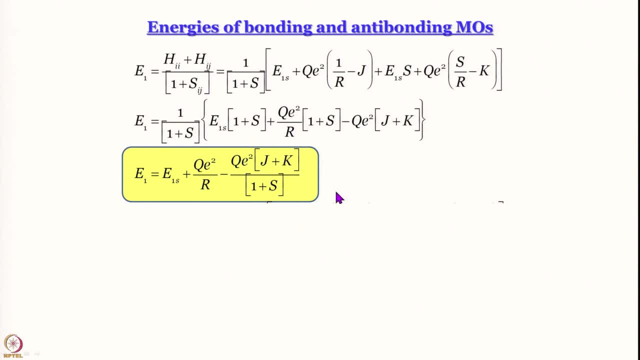 by 1 plus capital S. Similarly, you can work out an expression for E 2 and that turns out to be E 1 s plus Q, e square by capital R minus Q. e square into J minus k divided by 1 plus k. divided by 1 minus s. 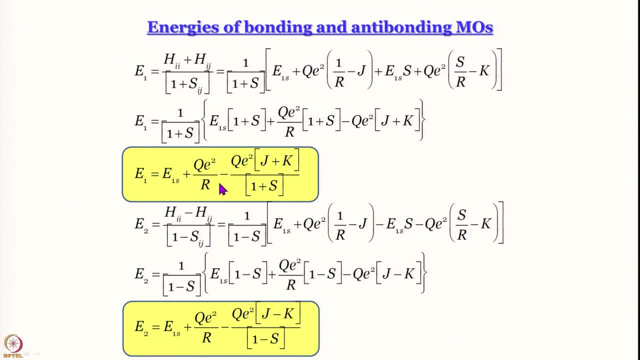 So see E, 1 s plus Q e square. what is that? that is simply energy of 1 s orbital plus the nucleus nucleus repulsion term. Q e square by r is the potential energy for nucleus nucleus repulsion. So this is the energy that we get if there is nothing else happening. okay, so 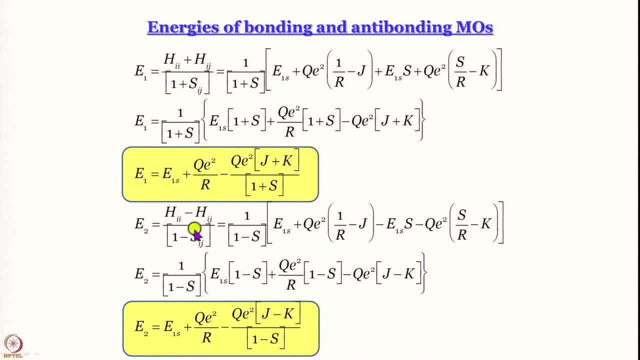 this is basically destabilization. This Q e square by r is capital R. so when you bring in the third term, Q e square into J plus k divided by 1 plus s, or minus. Q e square into J minus k divided by 1 minus s. 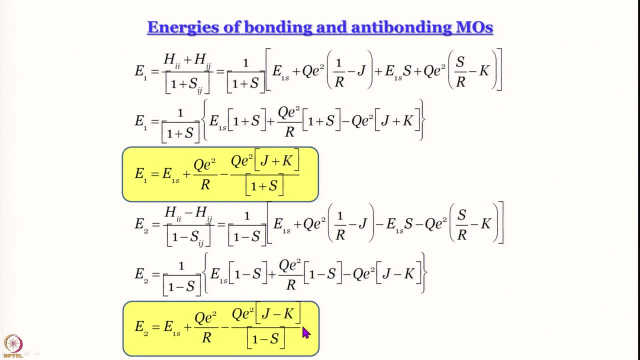 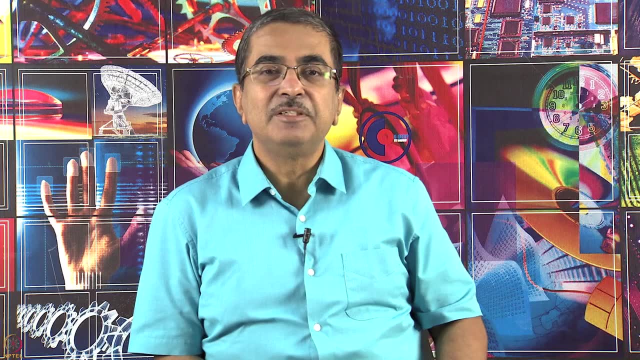 this third term decides whether you get net stabilization or net destabilization. So that depends on the integrals and remember, we are constructing these integrals using 1 s orbital to start with, But that will obviously not give me 1 s orbital. 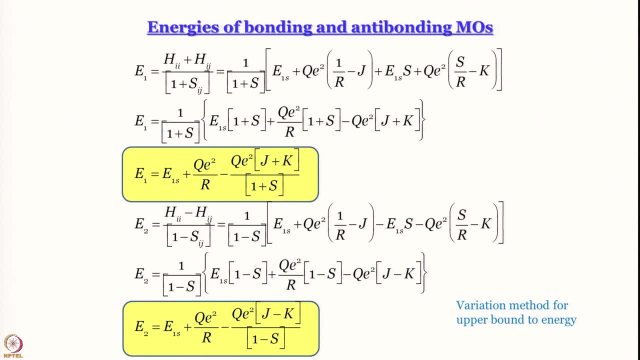 That will not give me very good result. So what is done is, as we have discussed, hydrogen type or by hydrogen, like orbitals, STOs, GTOs, in 1 s orbital expression, that Z is kept as a variational parameter, because here also you have two nuclei, right, you do not have a second electron yet, but that Z instead of. 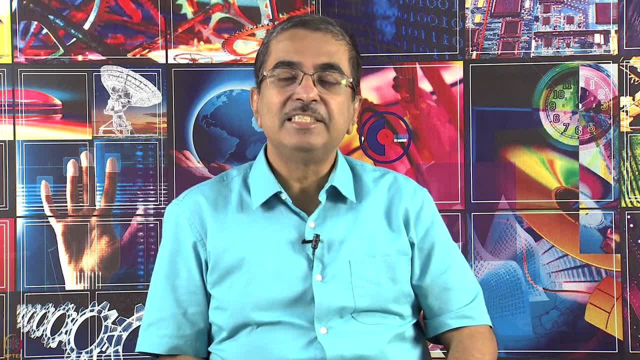 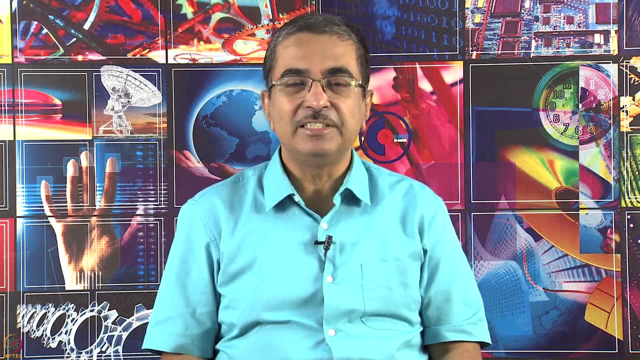 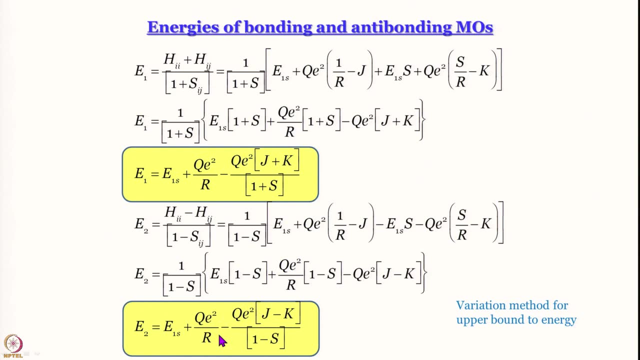 Z, you write Zeta variational parameter, So that is varied and you can also vary n And using variation method you can find the upper bound for the energies. that is how you find the expressions for E 1 and E 2 for given values of capital R okay. 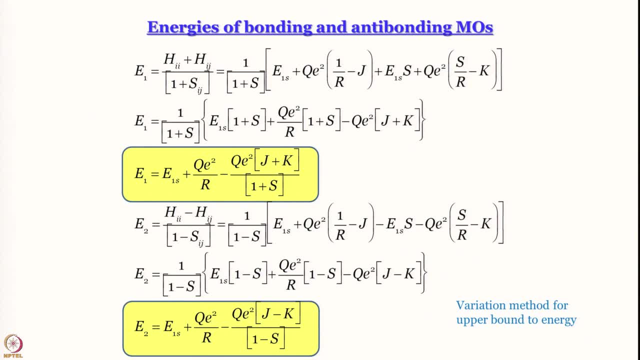 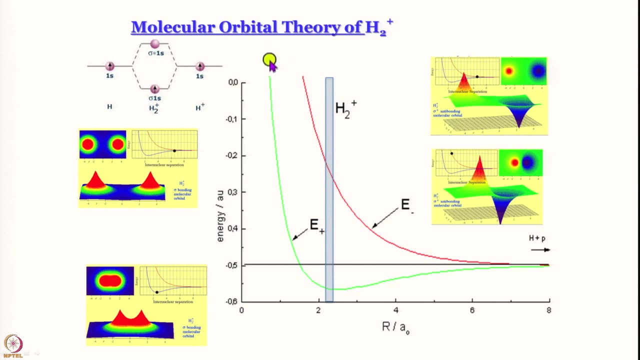 Another thing to remember is that J, k, s- these are also integrals that depend on the value of capital. R. okay, there is a very strong dependence of the energies and this is what you get. for E plus, You get a minimum and then it goes up. for E minus, it goes up all the way. 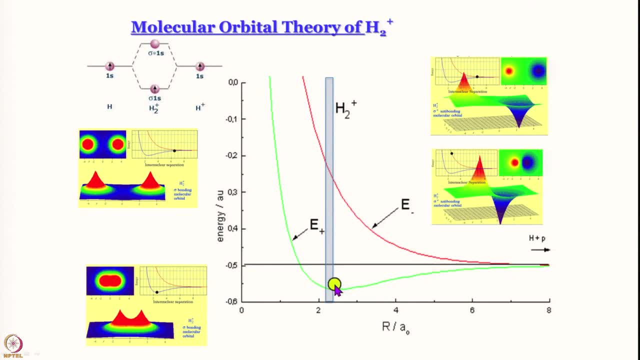 So this is how the energy of anti of bonding orbital varies as a function of R. this is how the energy of bonding orbital varies as ah of it is a bonding. anti. bonding orbital varies as a function of inter nuclear separation at equilibrium bond length. you can see that. 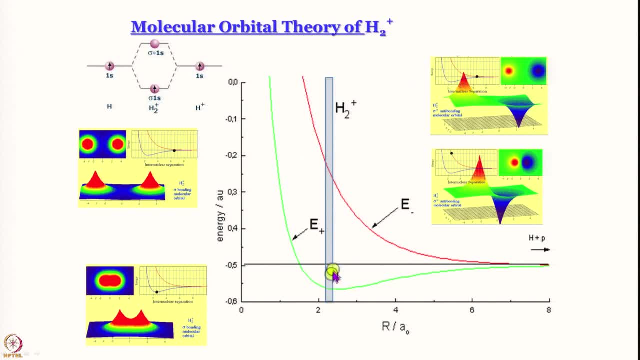 stabilization. the amount of stabilization that you have of the bonding orbital is actually less than the amount of destabilization that you have in the anti bonding orbital. So if you have 1 electron in bonding orbital, 1 electron in anti bonding orbital, since energy of the system will not be 0, it will be more than 0, right, and that is often explained by: 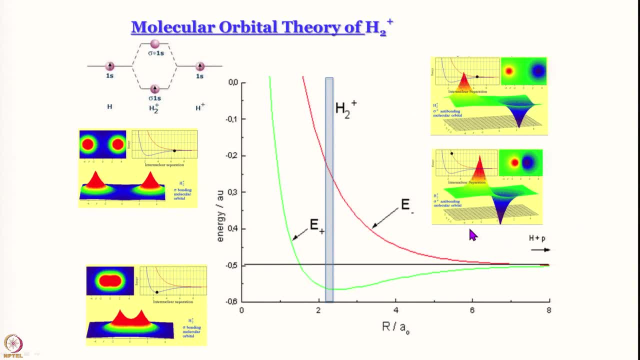 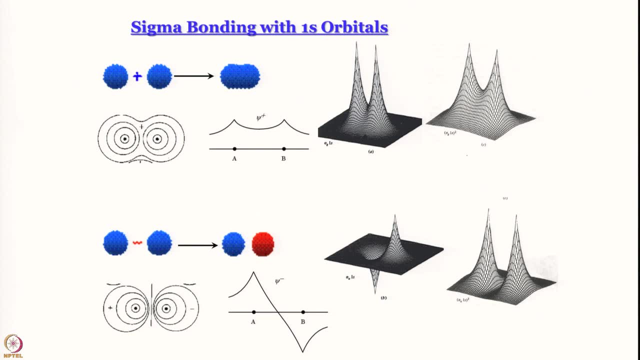 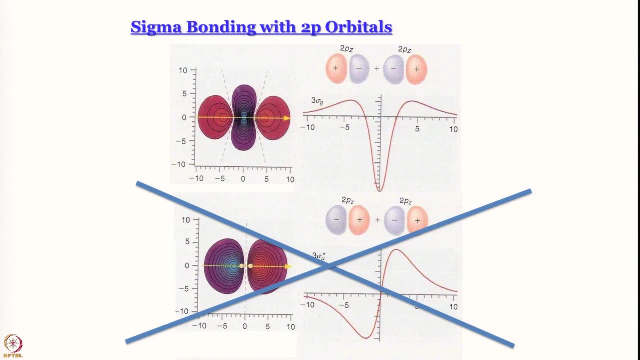 this hand waving arguments using this ah, this kind of orbital picture. okay, So we have already studied sigma bonding with 1s orbitals. I leave it to you To work out the ah, at least shapes of bonding and anti bonding orbitals using 2p orbital. 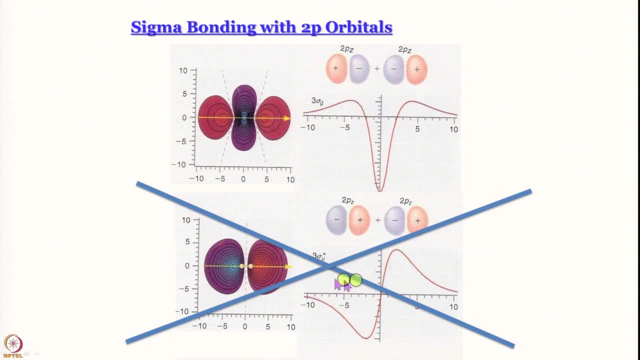 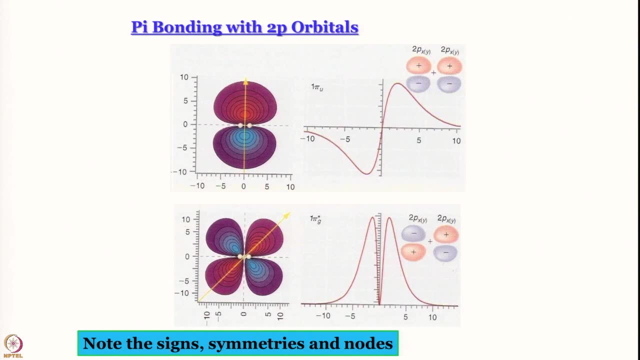 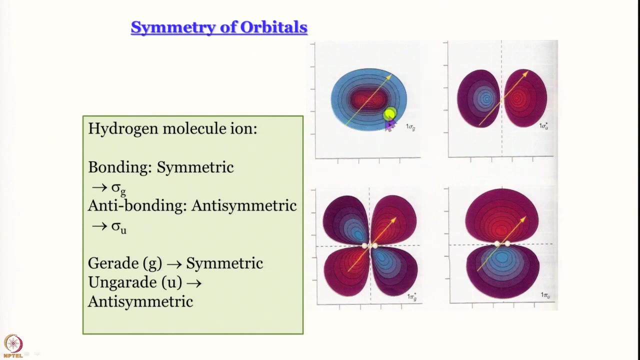 this is from ah, one of the textbooks- I have forgotten which one, but ah, this one is wrong. please do not look at that. And this is what you get for pi bonding using 2p orbitals. okay, just side on overlap. And one thing that you should remember or know, or understand is that symmetry of orbitals. 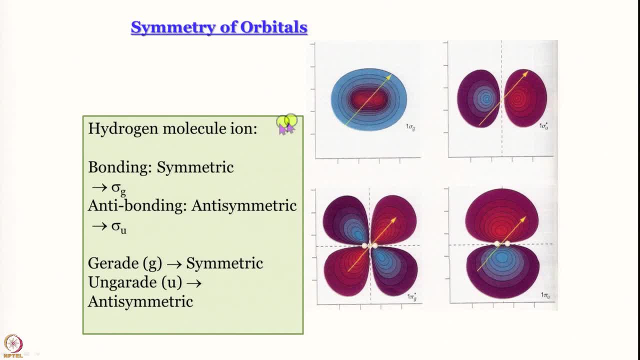 is often used as very important parameters For the hydrogen molecule ion for bonding orbitals. it is symmetric with respect to inversion, So it is called sigma g, g for Zeraday. The anti bonding orbital is anti symmetric with respect to ah inversion. that is called 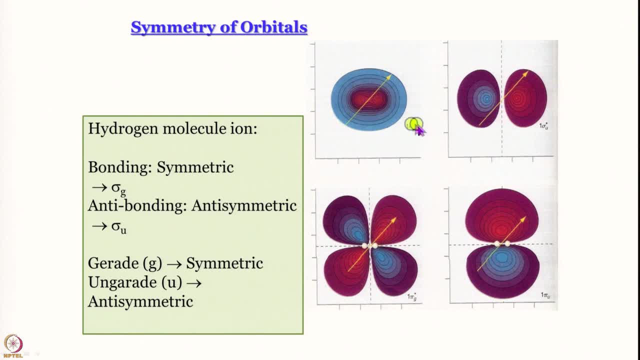 sigma. u do not think that always bonding orbitals are Zeraday and anti bonding orbitals are Zeraday. that is not the case. if you look at the bonding pi orbital used by ah side on overlap of 2p orbitals, You see that this bonding orbital for pi is 1 Zeraday and anti bonding orbital is actually. 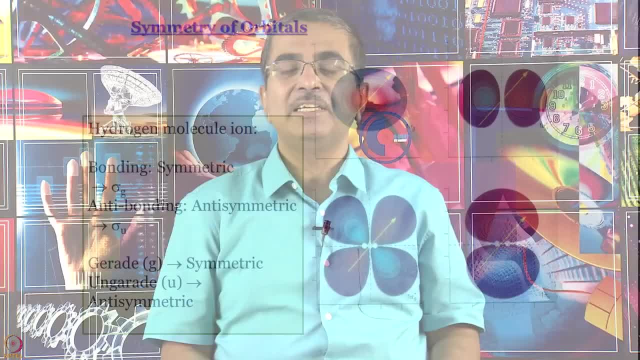 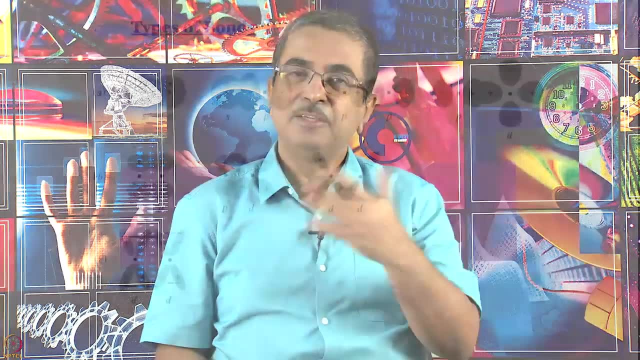 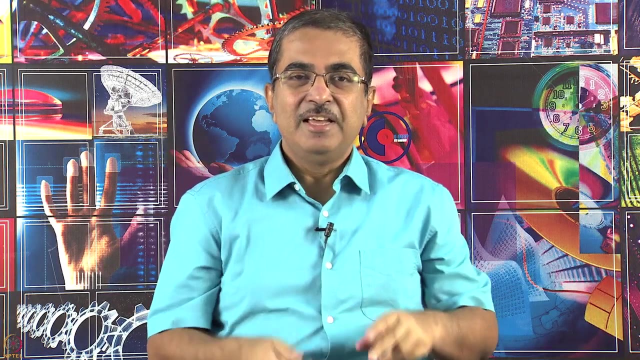 Zeraday. okay, So we are going to use this in the nomenclature of MOs when we talk about ah, actual molecules, And using this, I think you already know what are the types of bonds: sigma, pi, delta. okay, These are ah examples of what kind of bonds. 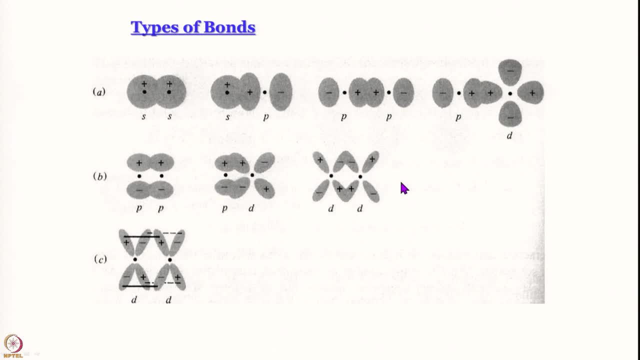 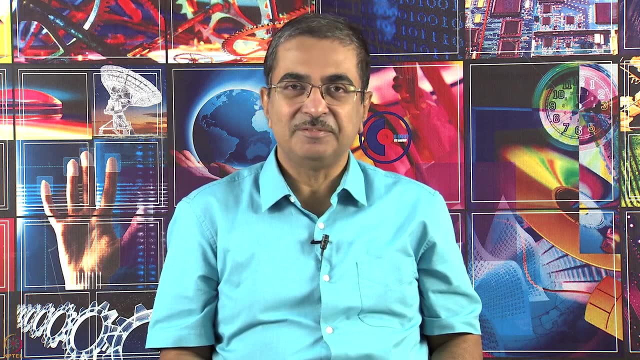 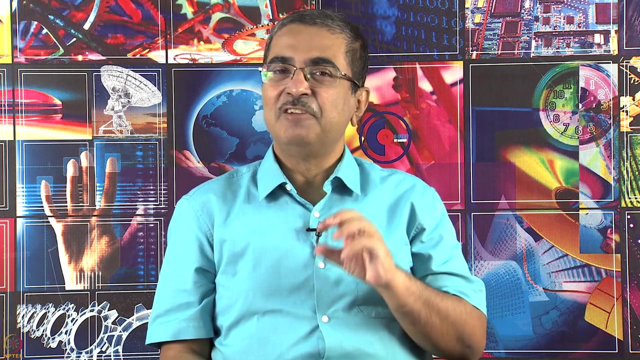 Bonds are formed using different orbitals. again, I leave this to you as an assignment. in case of any difficulty, any question, please feel free to contact us or ask in the open session. This completes our discussion of H 2 plus. ah, little longish, ah module. sorry, very fast. 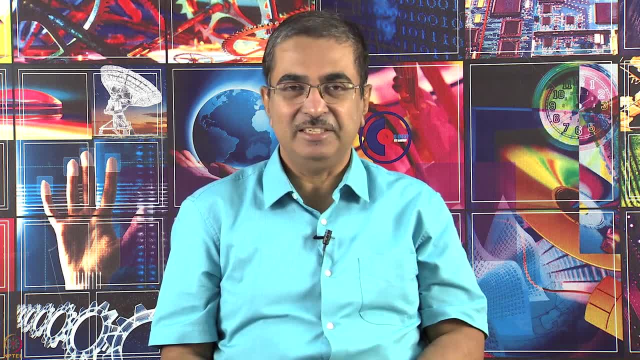 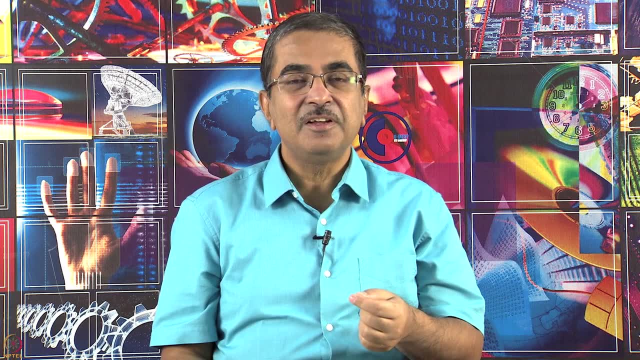 but it is a deputation of what we have done earlier. I am sure you will be able to handle it With this knowledge. we next discuss H 2 molecule. we bring in another electron and use the same orbital, perhaps with modification, for things like shielding.